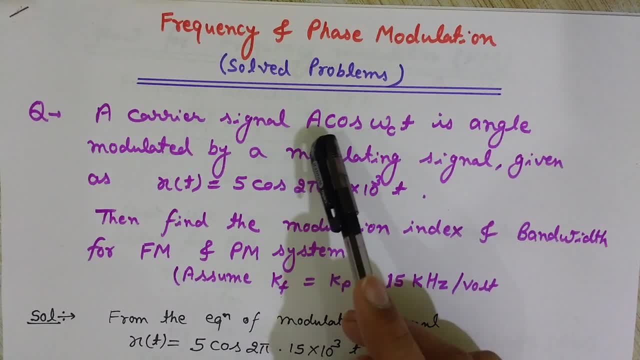 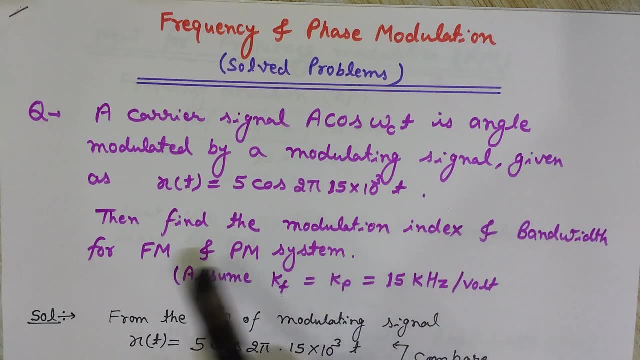 And this is the carrier signal, a cos of omega c, t, And I want to find the modulation index and bandwidth for both frequency modulation and phase modulation system. I am given here kf and kp equal to 15 kilohertz per volt. What is kf and kp? Actually, kf and kp, both are the proportionality constant and kf denotes the frequency modulation and p is for phase modulation. 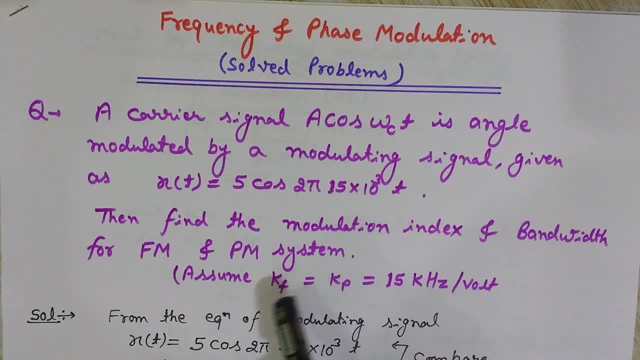 kf is what? kf is the frequency sensitivity of the modulator in frequency modulation and it is the phase sensitivity of the modulator in phase modulation. So it is also given as that these both are equal. So first of all, let's see some basics, like in this modulating signal. Modulating signal has been given message. signal is this. This is the equation, and I will compare this modulating signal with phase modulation. 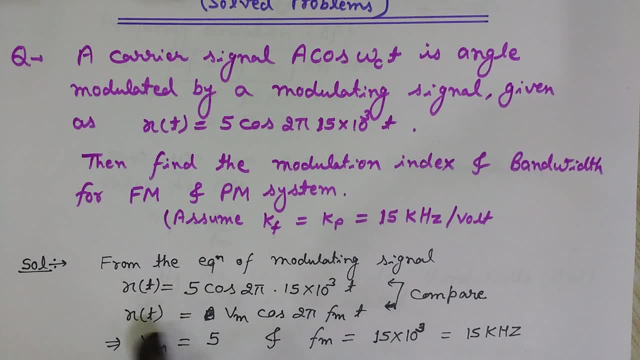 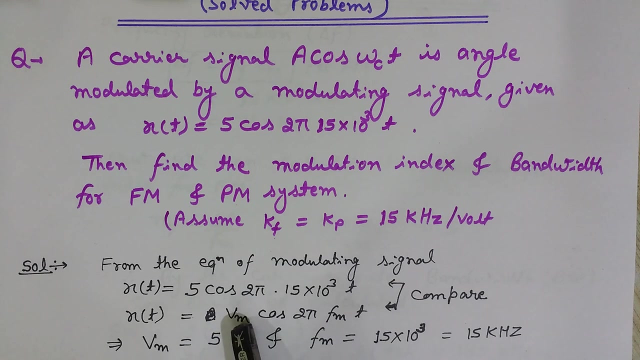 Modulating signal with the standard format of the modulating signal, x t is given as v m cos of 2, pi, f m, t. Here v? m is the peak amplitude of the modulating signal message signal and f? m is the frequency, the maximum frequency present in the modulating signal. If I compare both of these then I will see that 5 is the 5 is equal to the v m. I will see that v m maximum amplitude of the modulating signal is 5 and the frequency of the modulating signal is 5.. 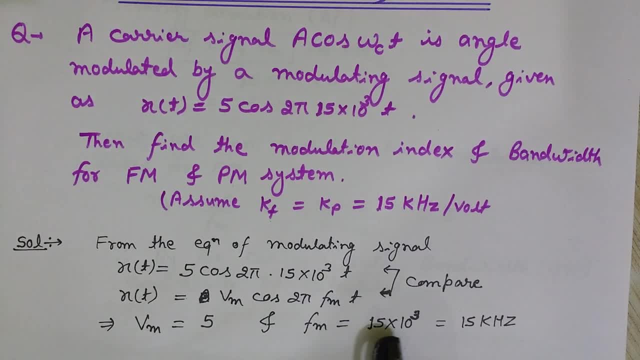 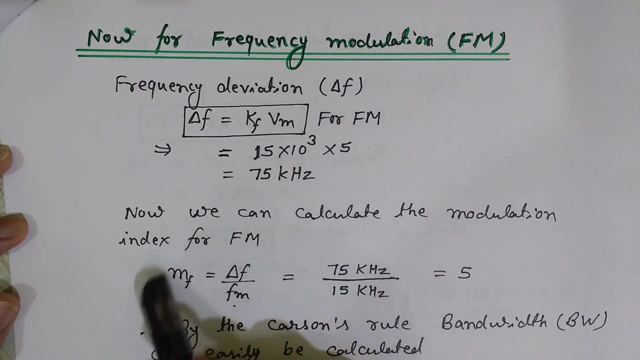 Component f m. the maximum frequency is 15 into 10 to the power 3, that is 15 kilo hertz. Now I know both of these things. My job is now to find the modulation index and the bandwidth for f m first. First we will see both of these things for f m, then for phase modulation. So let's see it. This is the case for frequency modulation. If I want to calculate the modulation index, then for modulation index. 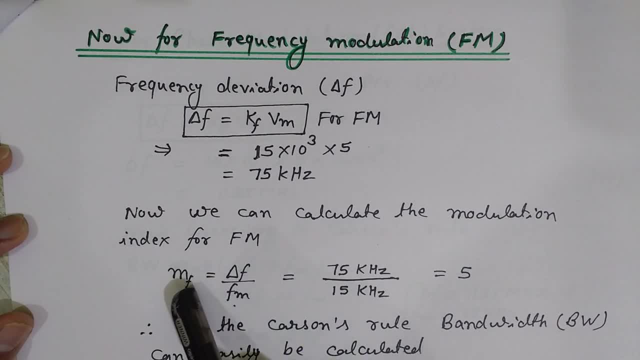 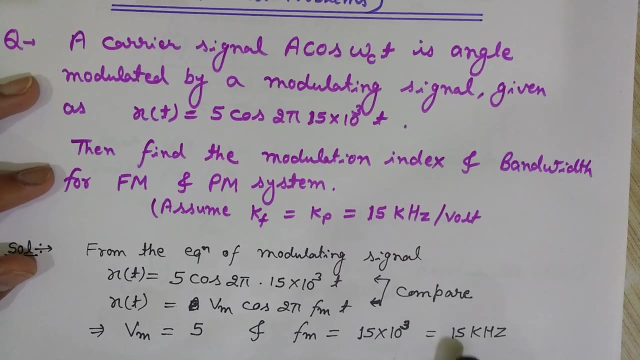 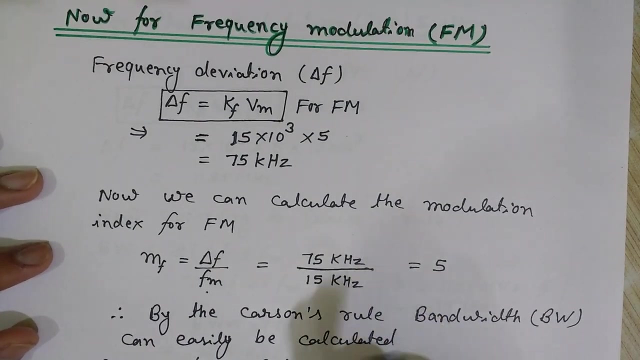 the formula is delta f divided by f m m. f is the modulation index for frequency modulation and delta f is the frequency deviation and the maximum frequency present in the signal. As I know that f? m is given to me 15 kilo hertz, I already know this, This 15 kilo hertz. I have already calculated f? m, but I do not know the value of delta f here. This is delta f, and for modulation index I need both of these. So 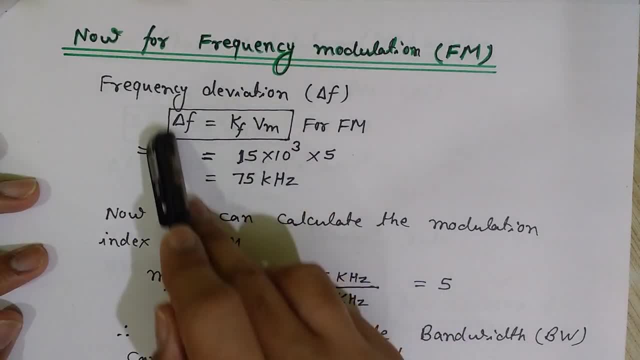 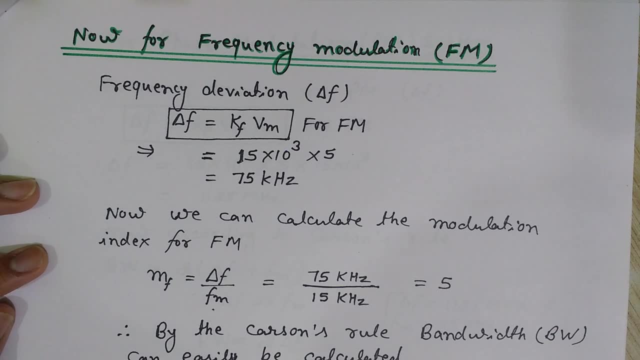 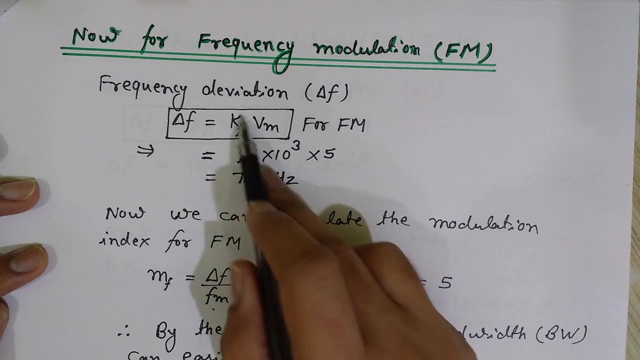 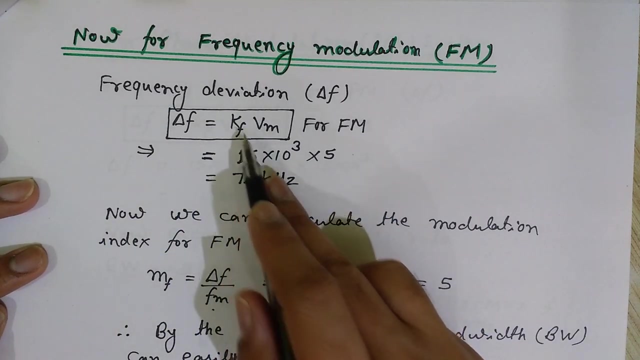 for delta f, the formula for frequency modulation. these formula are important. You learn it that delta f is equal to k f into v m. Delta f is equal to k f into v m, V m. I know maximum amplitude of the modulating signal and k f is also given to me, the proportionality constant or the frequency sensitivity of the modulator. k f is given 15 into 10 to the power 3.. We know that k f is given 15 into 10 to the power 3.. So we 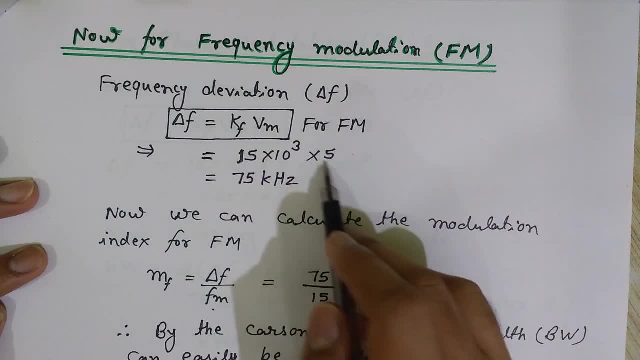 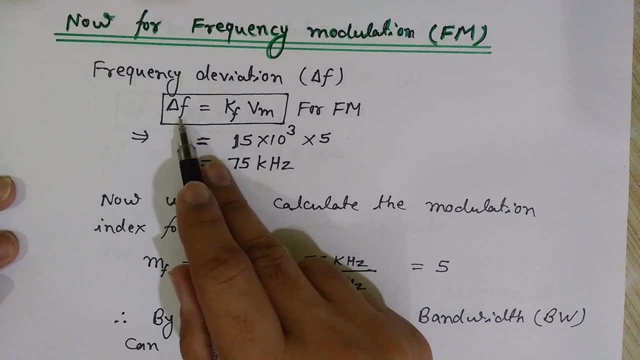 and kpr 15 into 10 to power 3 and vm is 5. okay, from here vm is 5 and kf and kpr 15 kilohertz. so i got the delta f as 15 kilohertz. now i can put this delta f at this place. so 75 by 15 is. 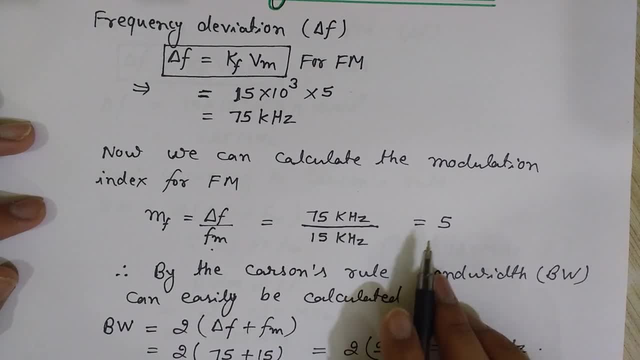 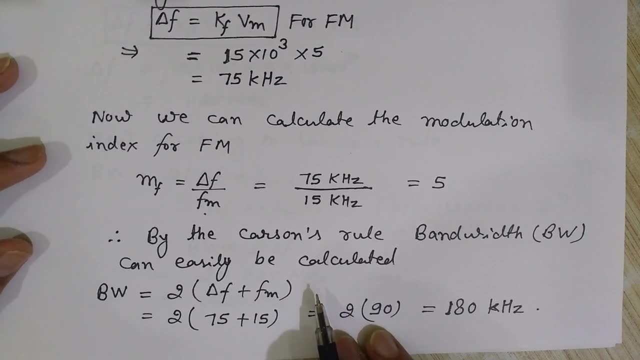 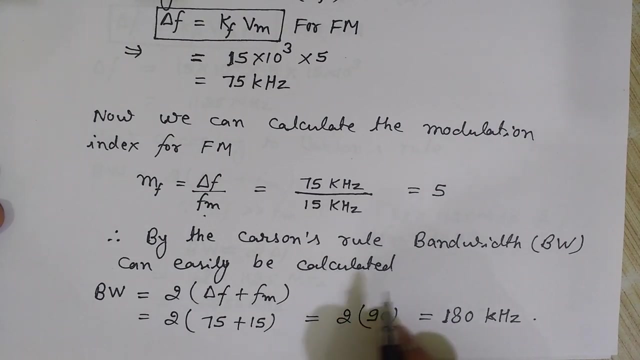 equal to 5, so 5 is the modulation index for frequency modulation. now i need to find the bandwidth for fm and by the carson's rule. if you don't know what is carson's rule, you can watch my video on carson's rule. okay, i will put the link in the description also. 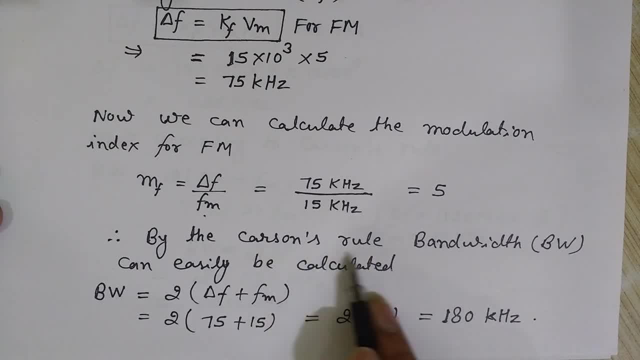 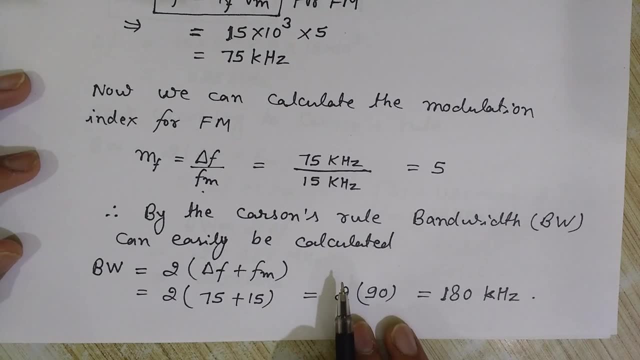 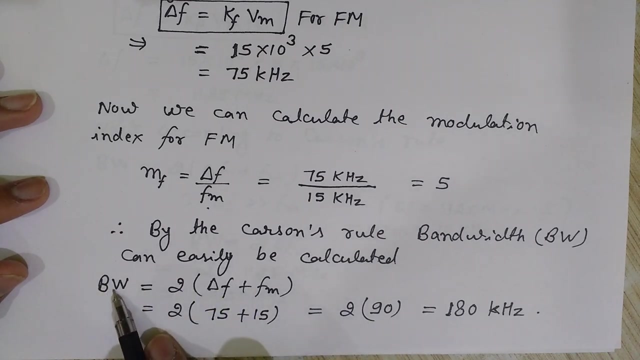 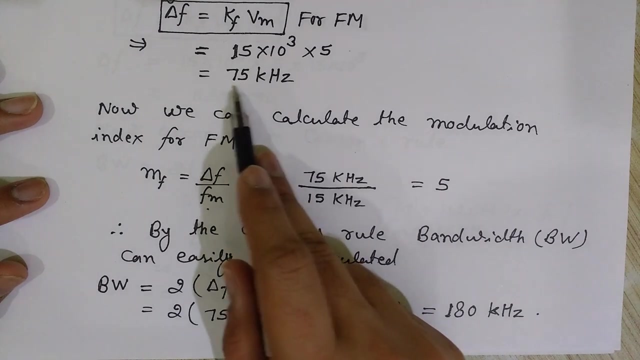 so you first understand what is carson's rule. but the formula, the main thing is the formula here, the rule. here it is. we can calculate the bandwidth easily if i have the delta f and fm. according to carson's rule, bandwidth can be given as two times of delta f plus fm. so here i have delta f, 75 kilohertz. okay, 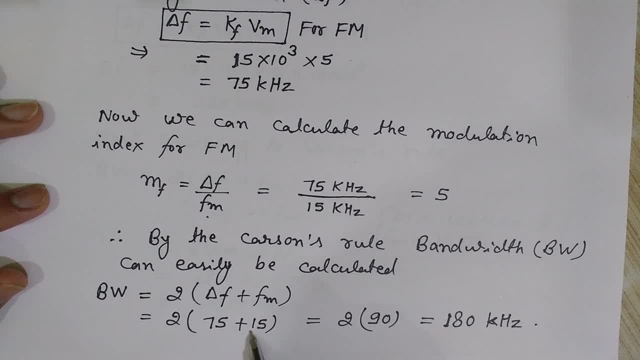 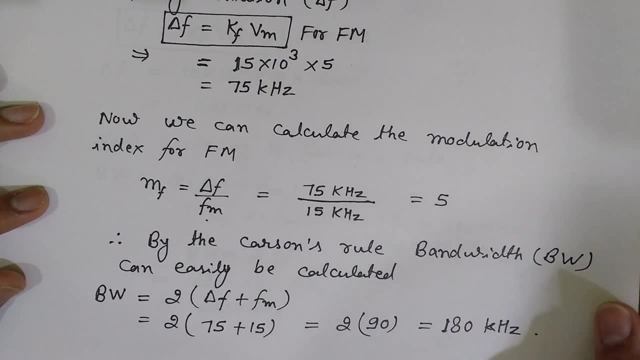 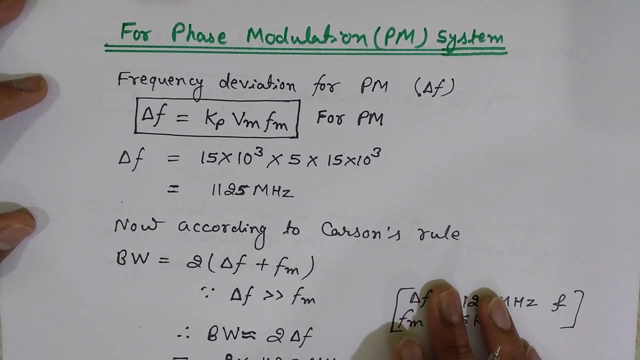 and also fm, so 15. so 2 times of 75 plus 15 is 180 kilohertz. so 180 kilohertz is the bandwidth for fm. now i have calculated the modulation index and bandwidth using carson's rule for fm. now i will show you how to calculate the bandwidth for fm. so i will show you how to calculate the. 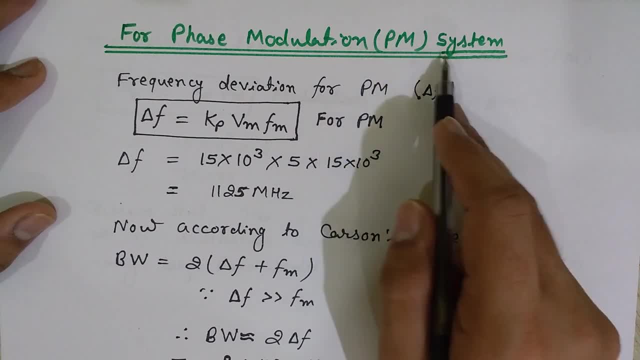 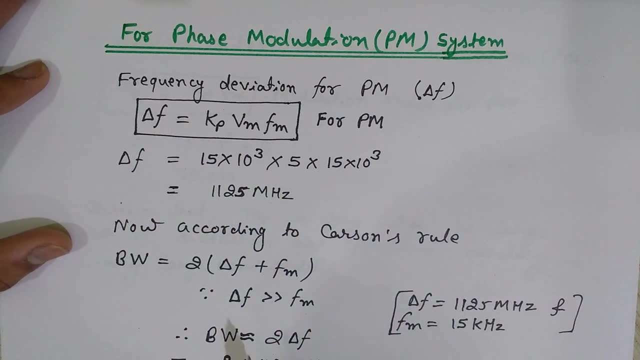 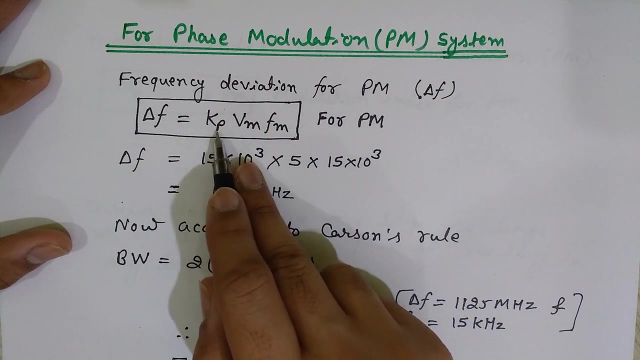 bandwidth for fm. so i will use- i will find both of these things for the phase modulation system. the formula are important here, so learn these formulas also. similarly, delta f- okay, delta f, the frequency deviation for the phase modulated system is given as kp into vm, into fm, which is 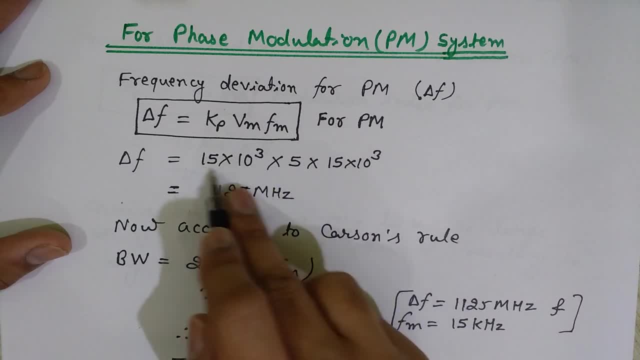 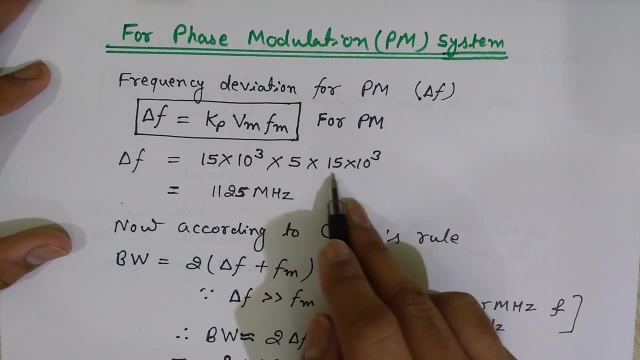 given, as which is already given to us: 15 into 10 to power 3, 15, okay, 15 to 10 to power 3, vm. vm is also clear. we know 5 and fm we also know. so 15 into 10 to power 3, we all know all these three things. so the delta f. 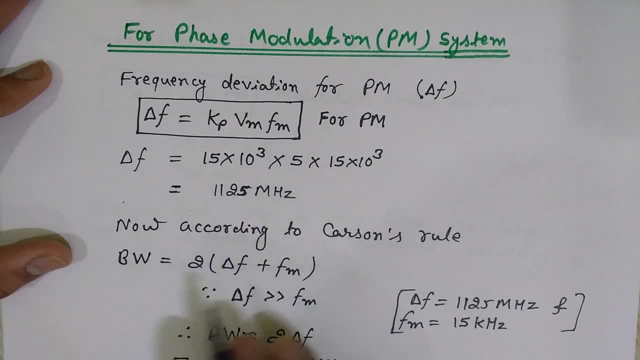 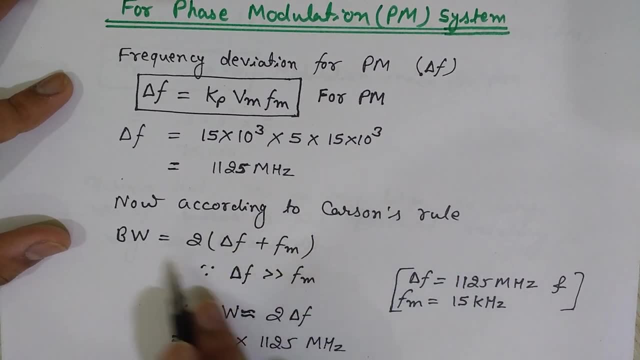 1, 1, 2, 5 megahertz, 1125 megahertz. okay, it is in megahertz now. according to carson's rule, we again apply the carson's ruler here. so bandwidth is given as two times of delta f plus f m, since 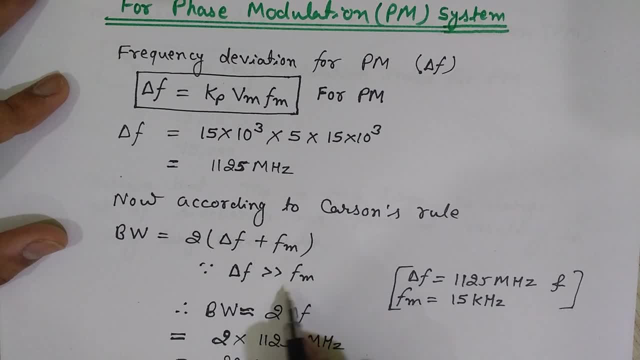 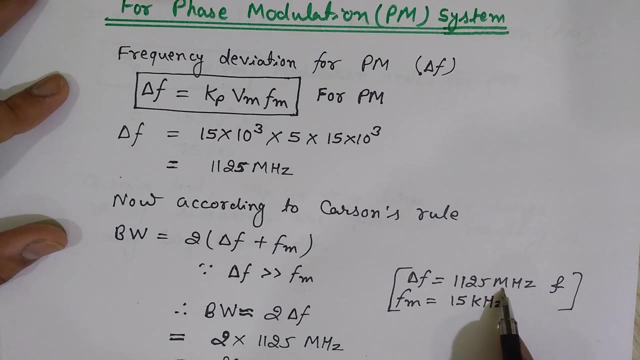 delta f is greater, greater than f m. how? because the delta f is 1001, 125 megahertz- we calculated just now, and fm is just 15 kilohertz. there is large difference. it is in kilohertz, just 15 kilohertz, and this is megahertz. that is also 1, 1, 2, 5. so delta f is 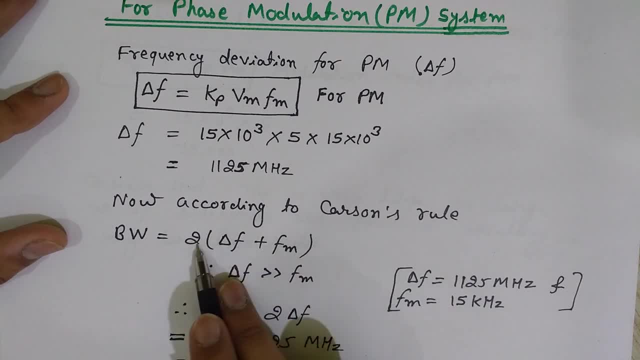 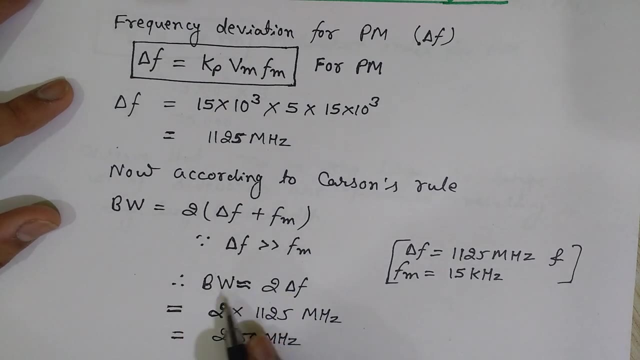 greater, greater than fm, so i can write this formula as i can neglect this fm in comparison to delta f. so this formula, delta f plus fm, can be written as simply delta f, so two times of delta f. so this approximate formula for bandwidth in this case is two times of delta f, so it is two into delta f is 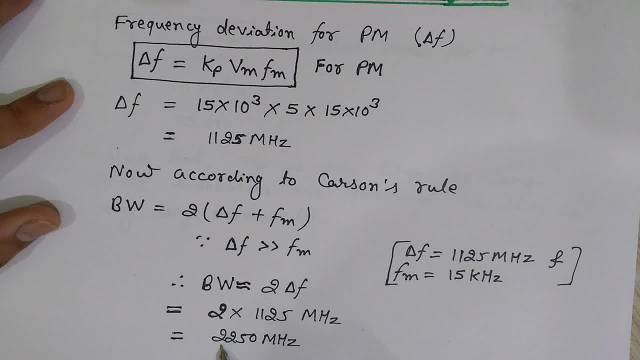 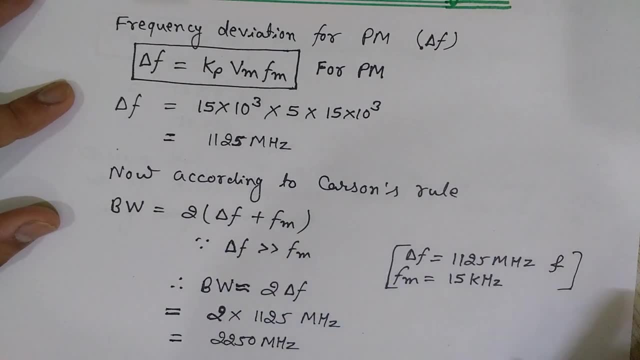 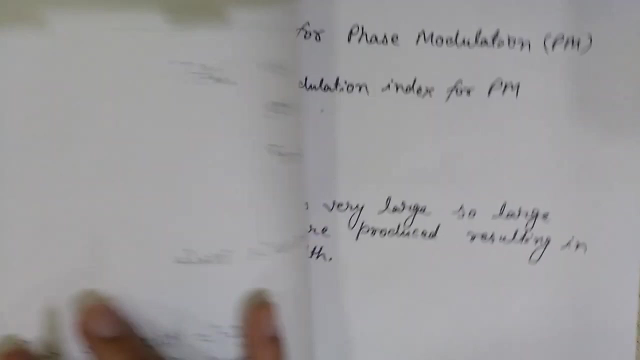 one, one, two, five megahertz. one one, two, five megahertz, which is 2250 megahertz. now we know the bandwidth for the phase modulation. now i will calculate the modulation index for the phase modulated system. it is the formula for phase, for the modulation index for phase modulation. 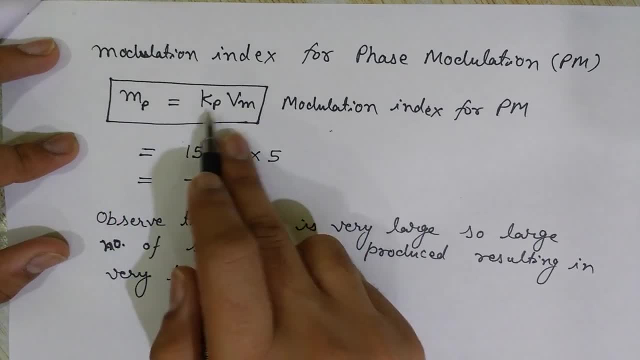 okay, it is given as kp into vm, kp. i know kp is 15 to 10, to the power 3 and vm is the 5. the maximum amplitude for the modulating signal is vm 5. so this is the formula for modulation index for phase. 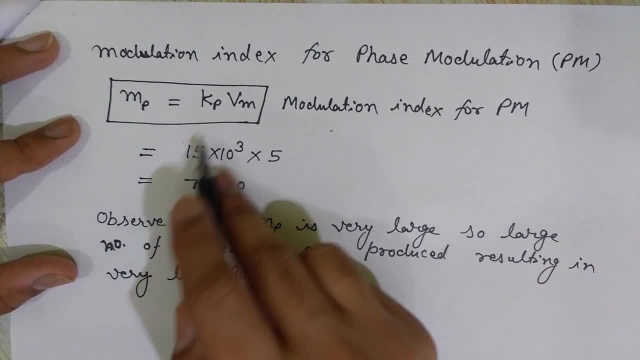 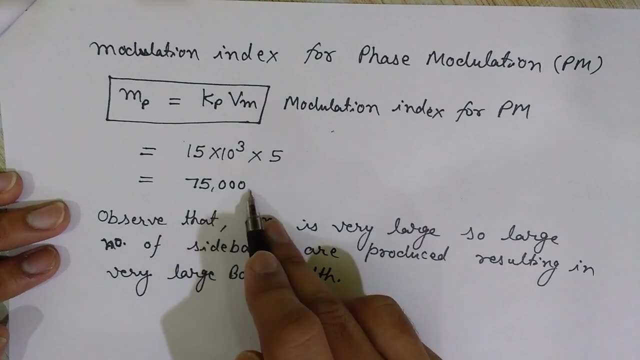 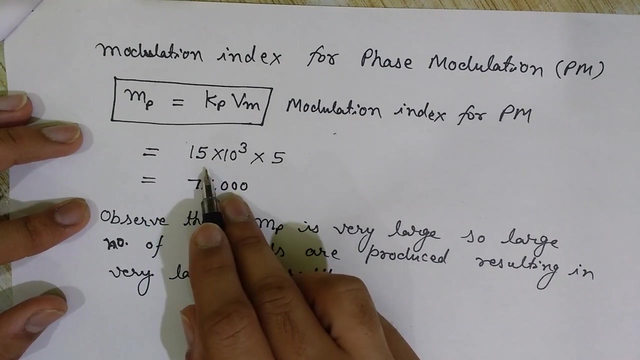 modulation. actually, you need to remember all these formulas. these all formulas are used here. so it is very simple. if i know kp and vm, it is 75 000. okay, it's a modulation index for phase modulation. here, this modulation index is 75 000, while the modulation index for the frequency 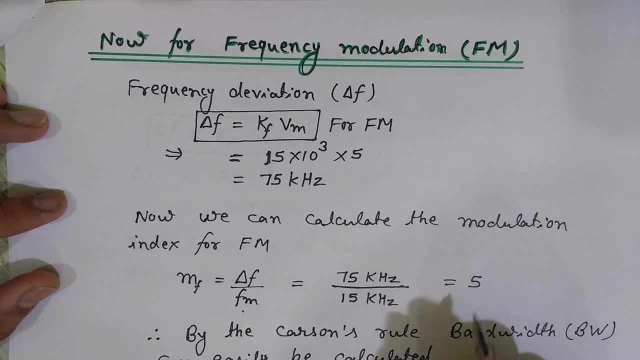 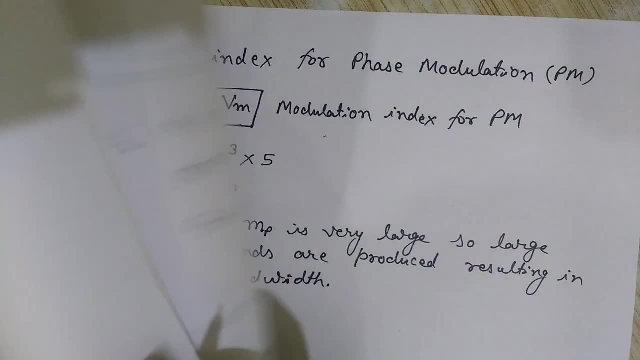 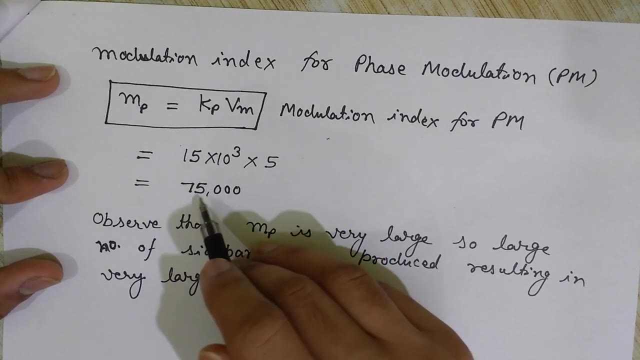 modulation was only 5.. so there is a very large difference between these modulation index of frequency and phase. here it is 5 and it is 75 000 here. so, because of this very large modulation index, we have large number of sidebands and these large number of sidebands. 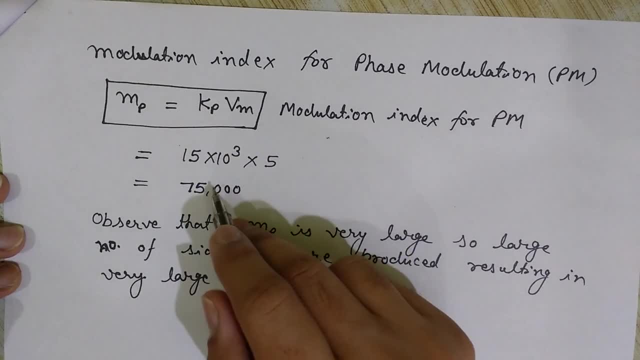 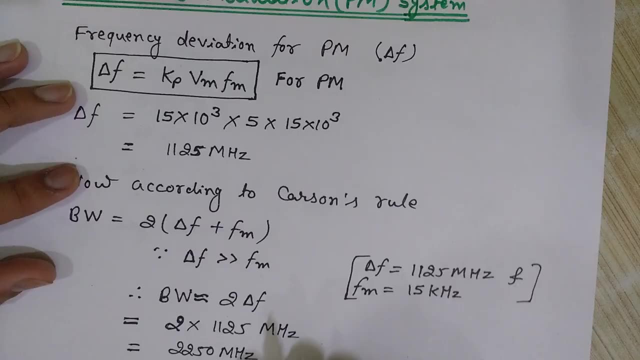 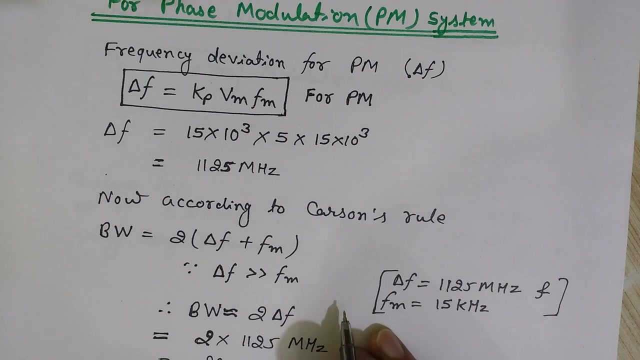 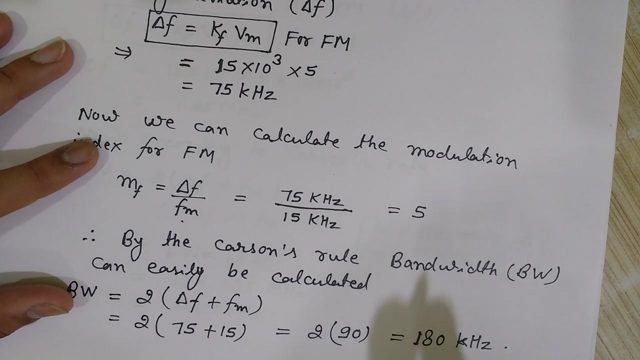 in very large bandwidth. okay, you have also seen that bandwidth is also larger in comparison to the frequency modulation. look at this: the bandwidth is 22 250 megahertz for phase modulation, while it was just 180 kilohertz for the frequency modulation. so this is large difference between this bandwidth. 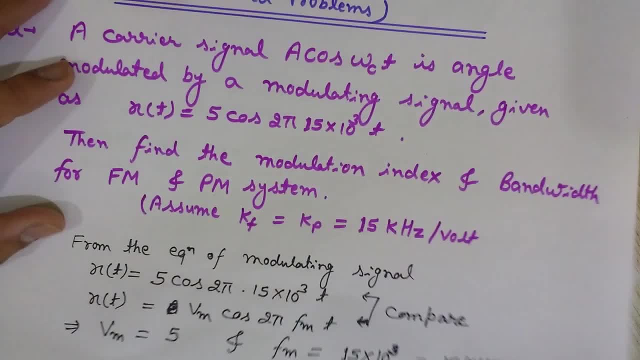 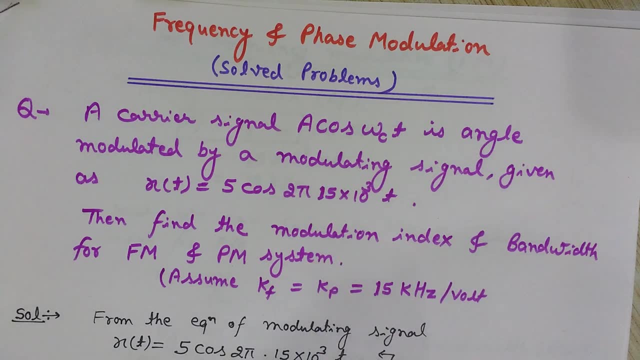 okay, so, so. so this was about the frequency and phase modulation. we learned how to find how to calculate the modulation index and bandwidth. if i have been given with the modulating signal equation, okay, we can easily calculate rule to calculate the bandwidth. okay, so i hope you got some information and like this video. 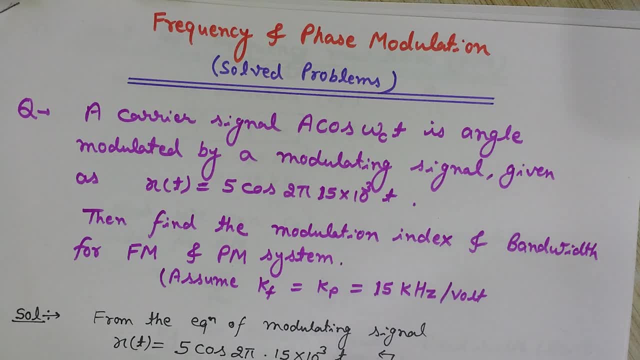 and, if you liked it, please click on the like button and share it with your friends so that they can also watch the video, and please do not forget to subscribe the channel. engineering made easy for more such informative and useful videos. thank you for watching. have a nice day, take care. 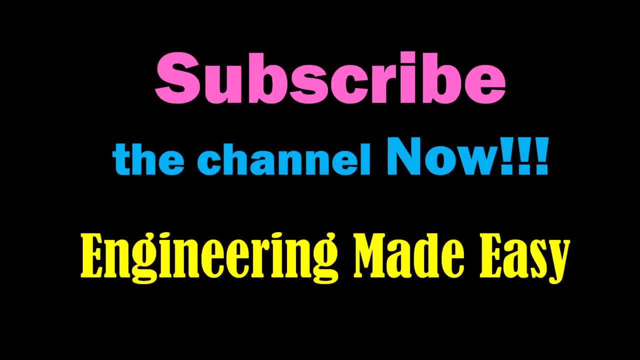 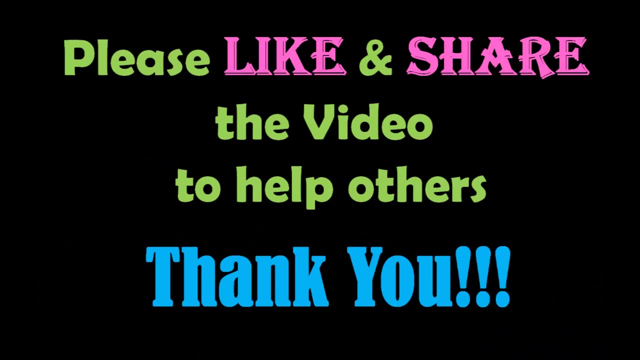 bye, friends. for more such videos you can subscribe my channel- engineering made easy- and please don't forget to like and share the video if you liked it. for more detailed information, you can visit my blog. see you soon in the next video. till then, bye.